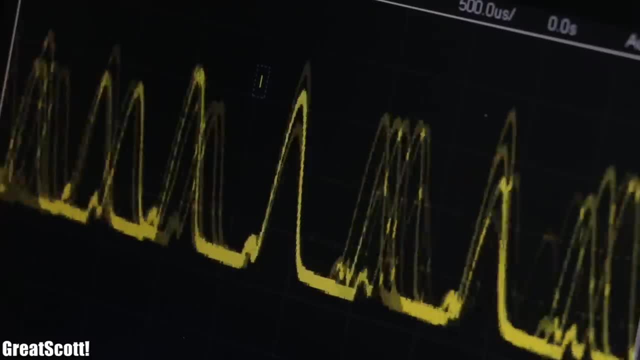 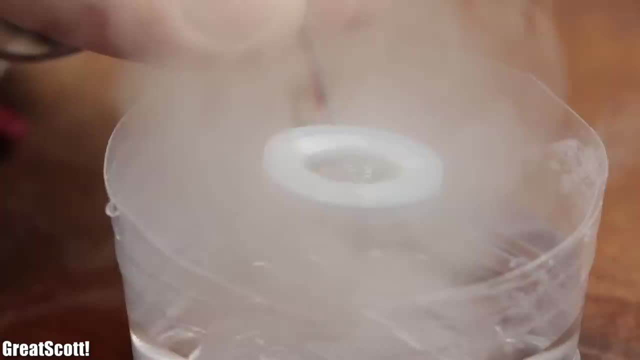 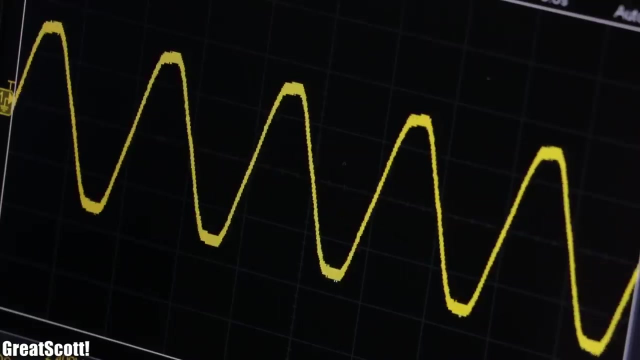 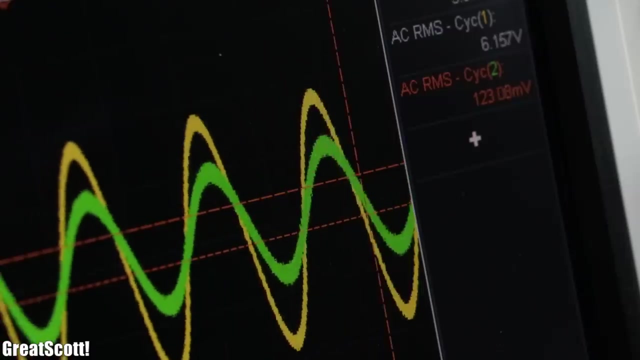 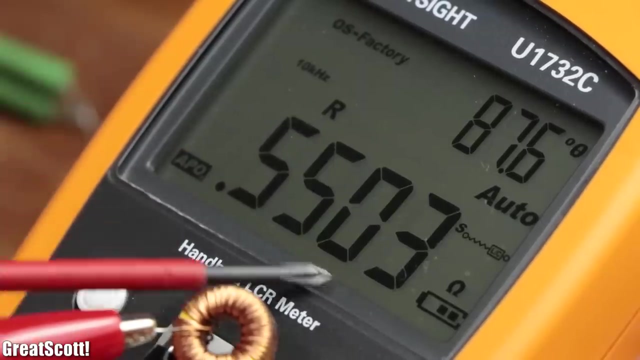 Unless, of course, we talk about switch-on. But DC is not almighty. While looking around us, we can see tons of applications where we got AC voltages, Most importantly our sinusoidal mains AC voltage. So in this video I will tell you about the basics of impedance, which, in a nutshell, is the concept of resistance extended to AC circuits, where now inductors and capacitors play an important role as well. 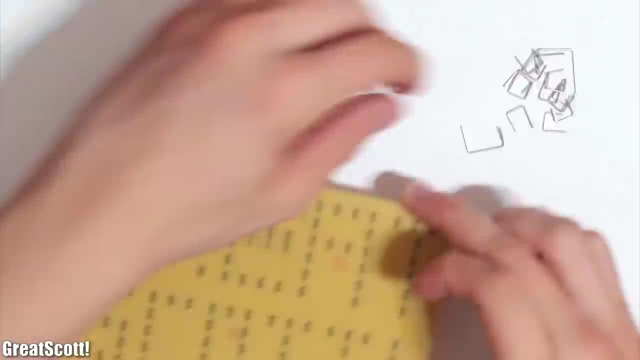 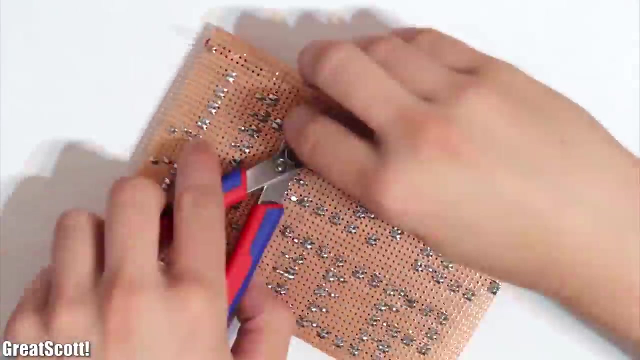 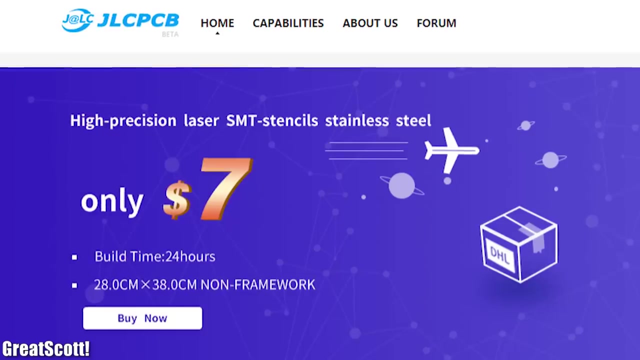 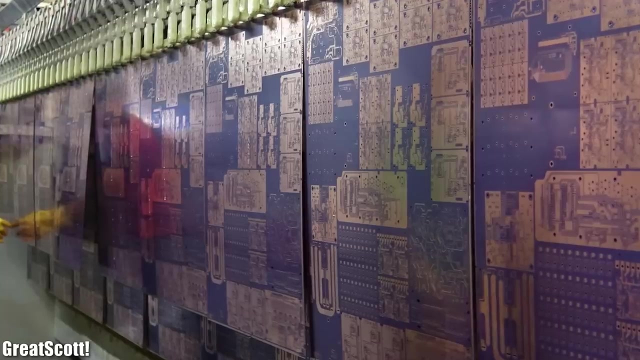 Let's get started. This video is sponsored by JLCPCB. One piece of news about them: JLCPCB will shorten the lead time of green 2-layer standard PCBs in the near future, So feel free to test out their PCB quality. 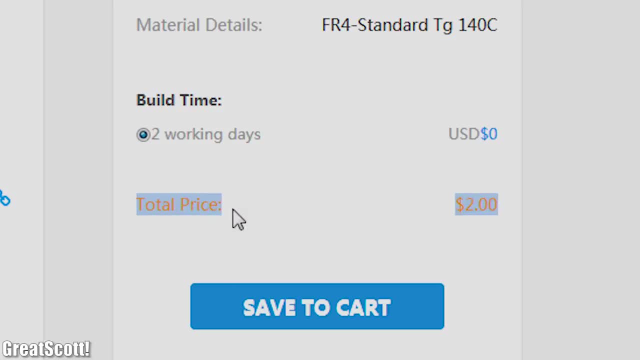 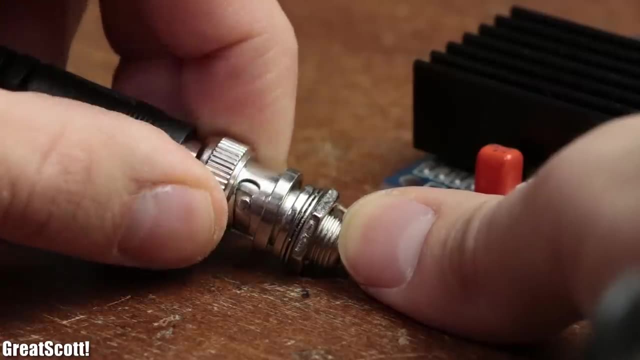 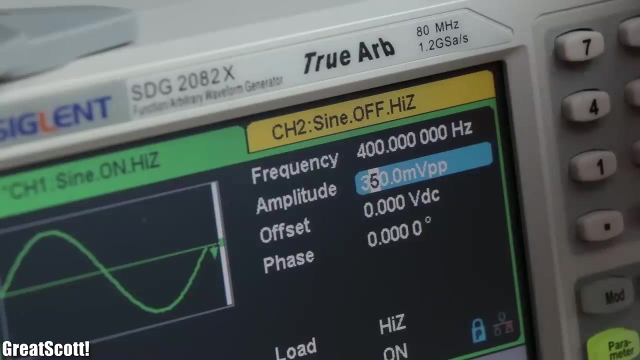 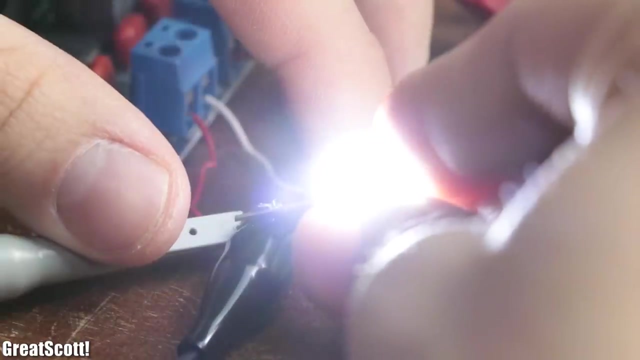 And fast delivery speed for a low price. For the experimental setup I connected my function generator outputs to the input of an amplifier. This way, by varying the frequency and amplitude of the function generator sine wave, I get the amplified sine voltage at the output of the amp that can handle a much higher power output. 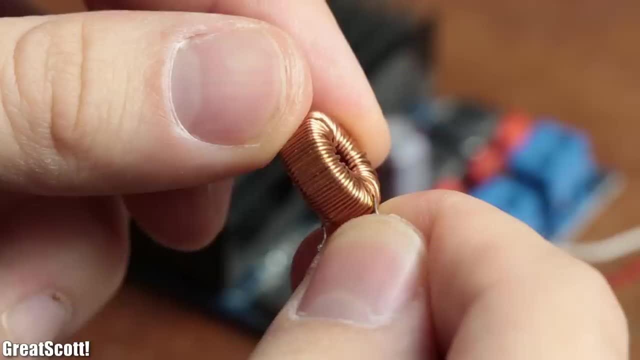 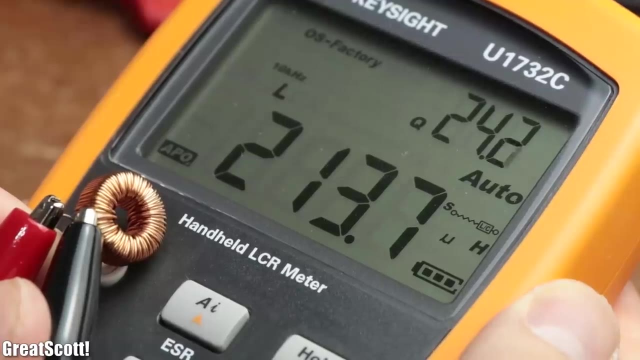 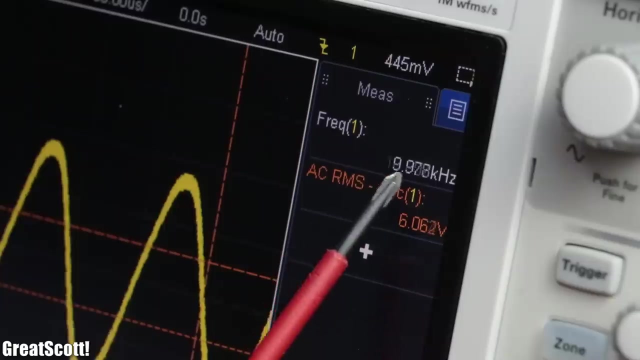 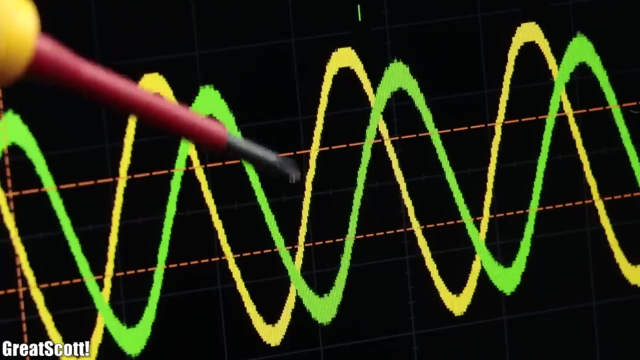 Which means we can know components up to it. For starters, let's use this small inductor, which features an inductance of around 214 microhenry, By connecting it directly to the sine wave, which features an RMS voltage of 6 volts and a frequency of 10 kilohertz, and observing the occurring current flow with a current clamp, we can firstly see that the voltage wave is leading, in comparison to the current wave, with a phase shift of around 90 degrees. 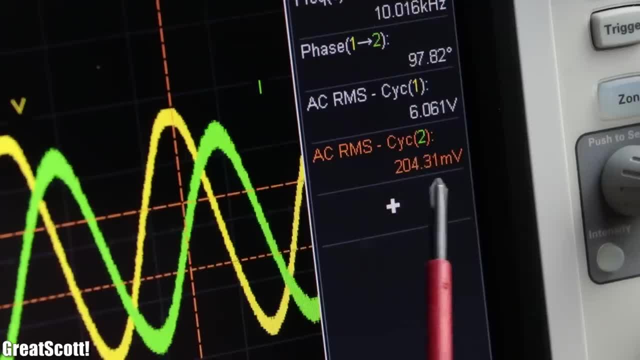 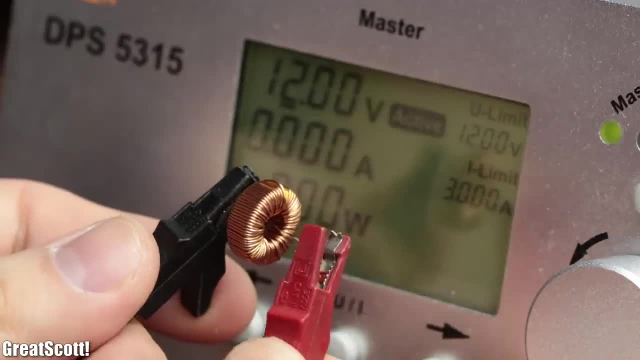 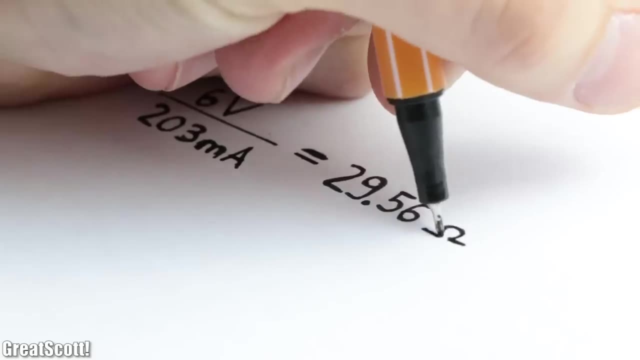 And also that an RMS current of 203 milliamps is flowing. That means that this time, the inductor does not create a short circuit like it did with DC. It resists the current flow just like a resistor would do, And thus this value is measured in ohms as well. 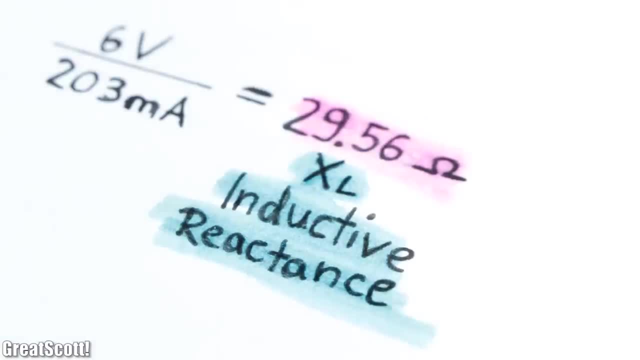 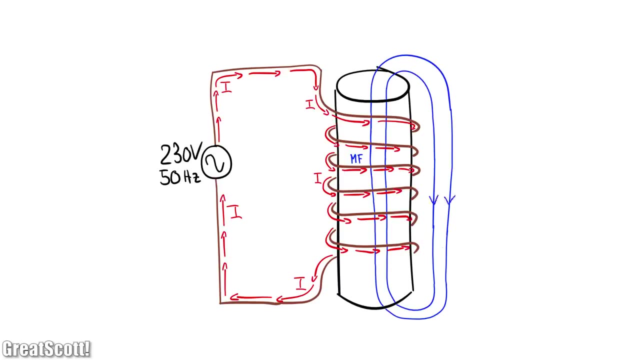 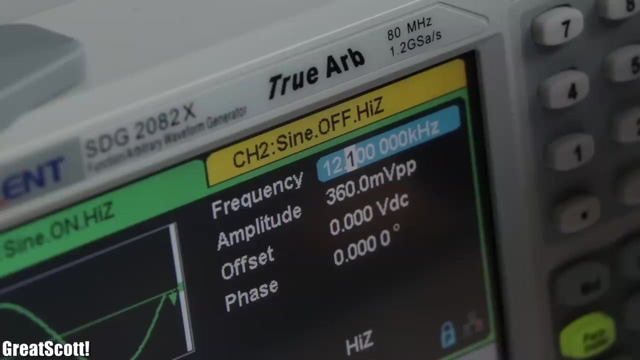 And is called the inductive reactance. This new kind of resistance originates from the fact that the constantly changing magnetic field of the inductor opposes the current flow, Which is also the reason why the voltage is leading with a phase angle, And by increasing the frequency of the sine voltage we can see how the current ohms value slowly decreases. 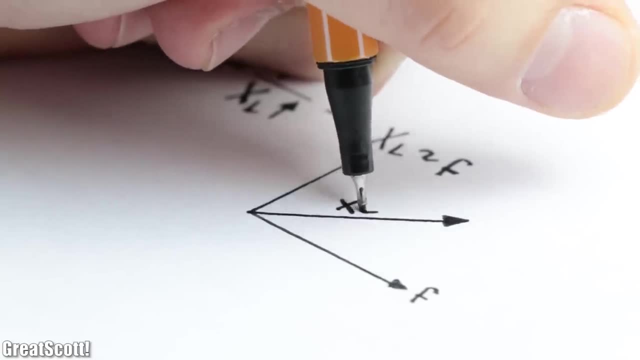 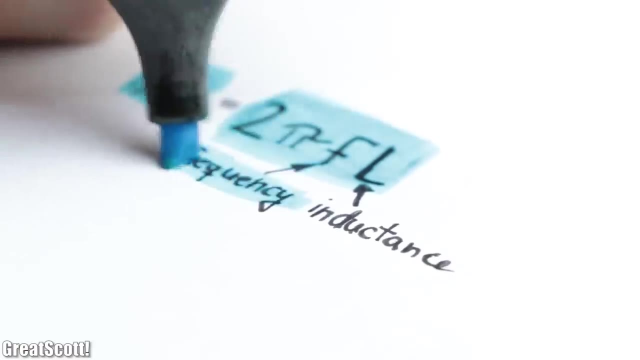 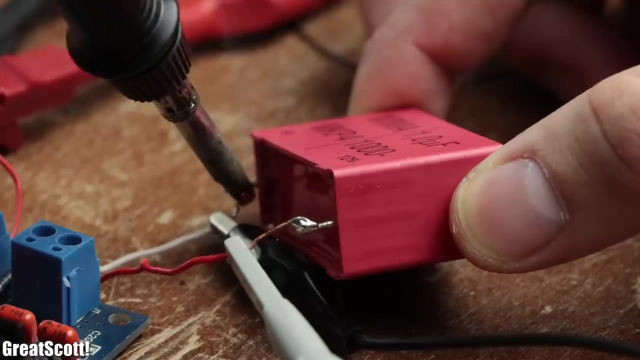 Which means our inductive reactance increases with the frequency. The final equation for it is 2 pi FL, With the frequency and inductance being the most important variable values. Now, if we would replace the inductor with a capacitor which features a capacity of 1 microfarad? 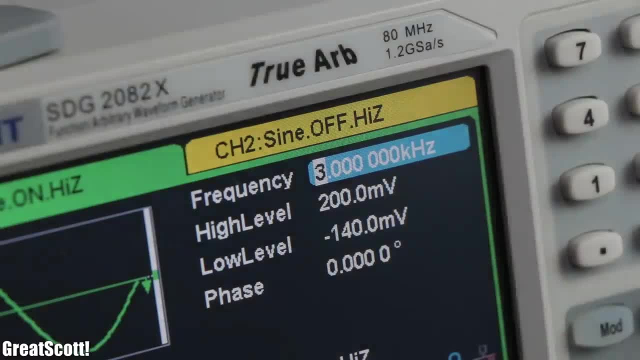 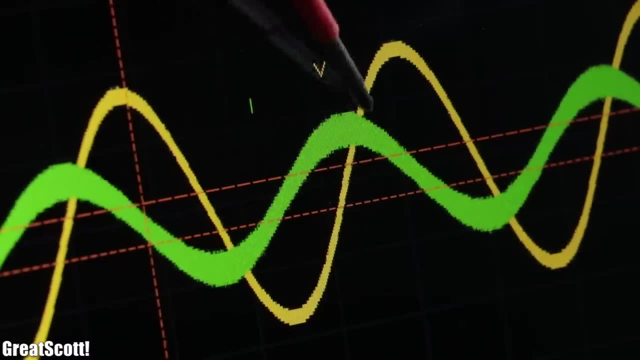 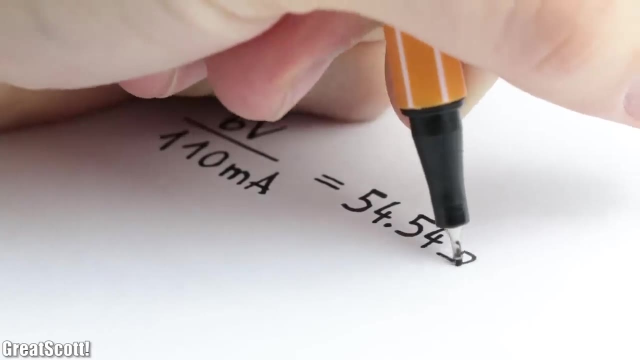 and use a frequency of 3 kilohertz, we can once again observe a phase shift of around 90 degrees, But this time the current is leading. Also, we got an RMS current flow of 110 milliamps, Which means just like with the inductor. 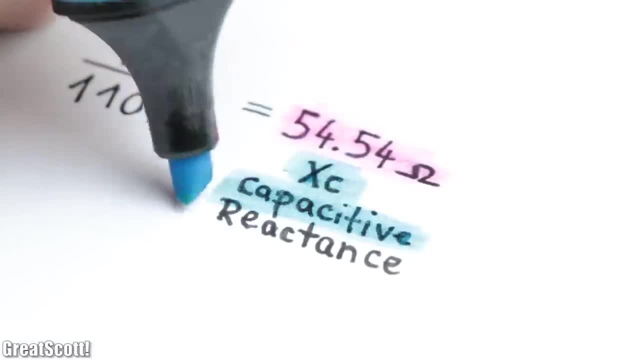 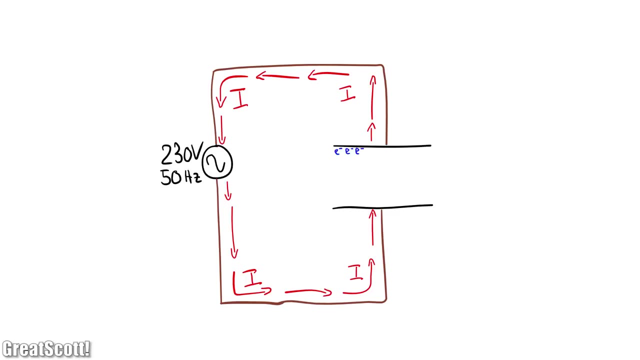 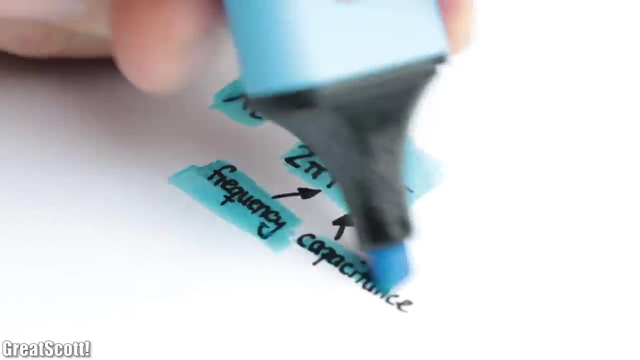 we got a new sort of resistance, This time known as capacitive reactance. Its cause is the constant charge reversal of the electrostatic field of the capacitor, And its equation once again features the frequency and capacitance as the most important variable values. 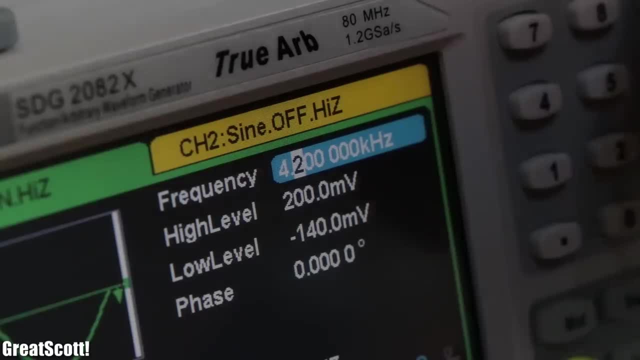 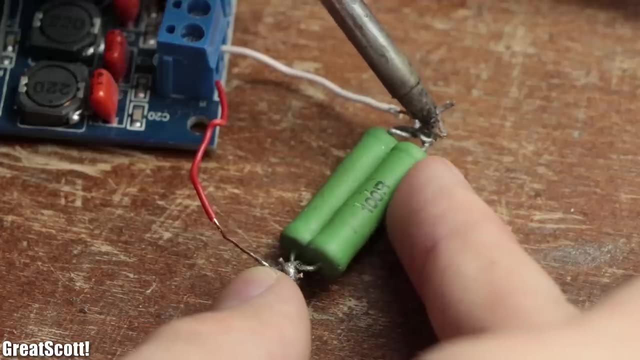 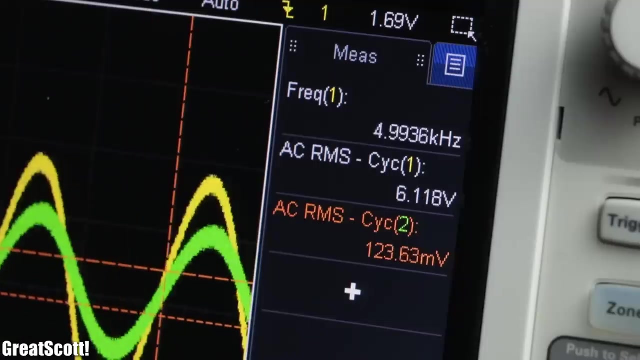 This time, though, with higher frequency, the current flow increases, Which means the capacitive reactance decreases. Now, if we go back to the plain old resistor and hook it up, we can see that it does not create a phase shift and its resistance, and thus current flow. 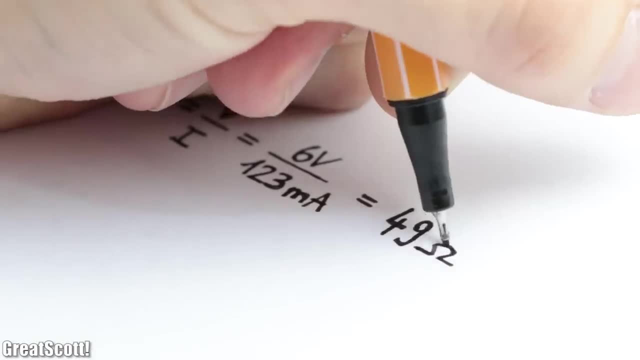 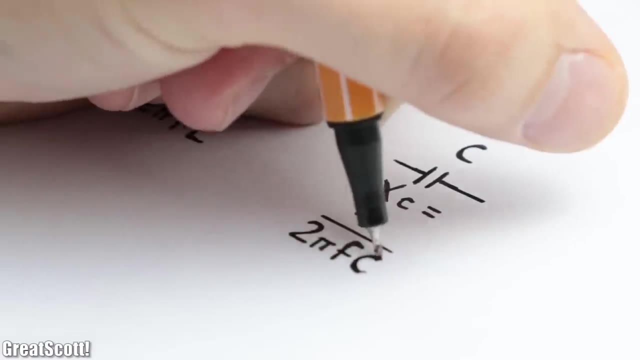 is not dependent of the AC frequency, It still only got its ohmic resistance. And just like that, you are now familiar with the reactance of the inductor and capacitor, Which not only changes the magnitude of the current flow dependent of the frequency, 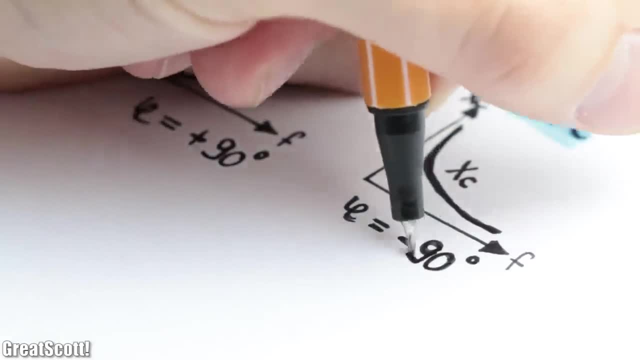 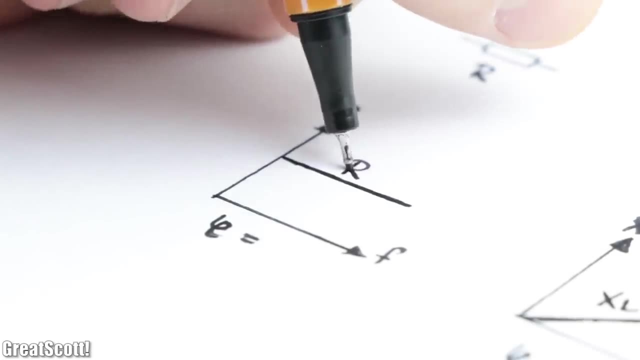 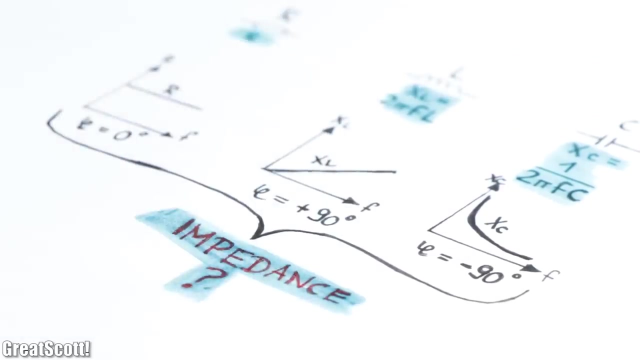 but also effects the phase angle between voltage and current. And of course we still got our ohmic resistance, which only influences the magnitude and not the phase. But the question remains: what does all of that have to do with impedance? Well, let's imagine we put a 50 ohm resistor. 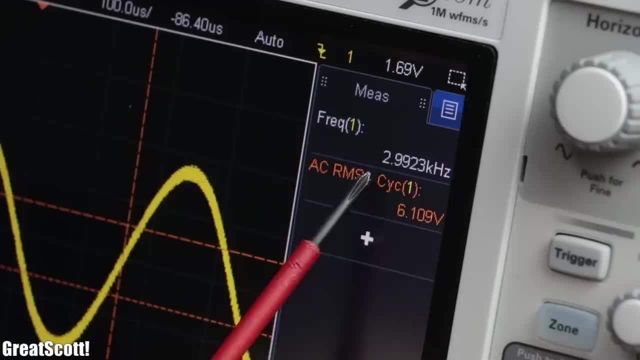 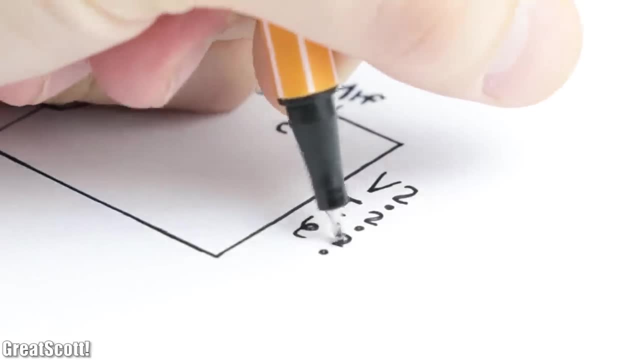 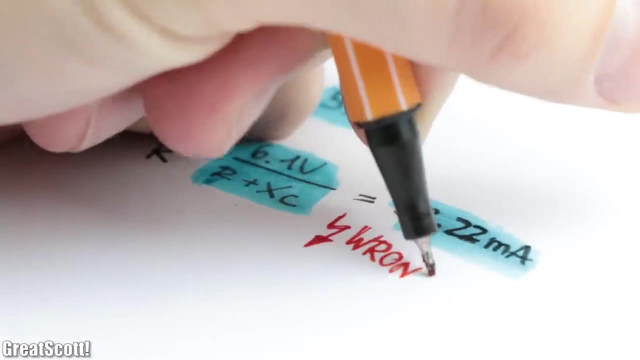 and a 1 microfarad capacitor in series to the 3 kilohertz 6.1 volt sine voltage. How can we calculate voltage, Current and phase angle values? Simply adding the ohmic resistance to the capacitive reactance and calculating with that. 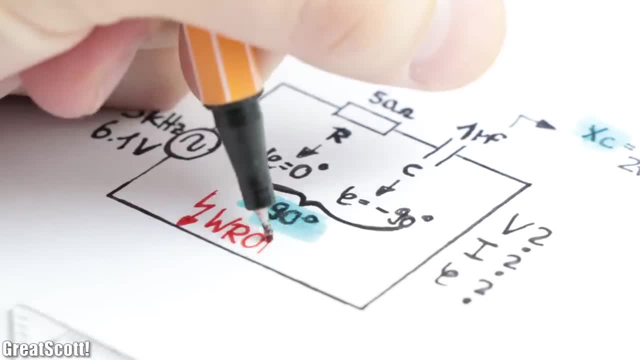 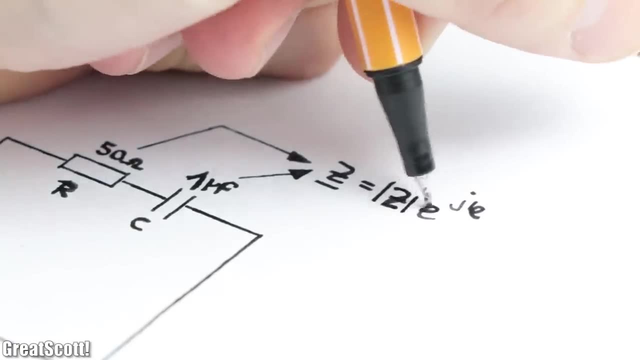 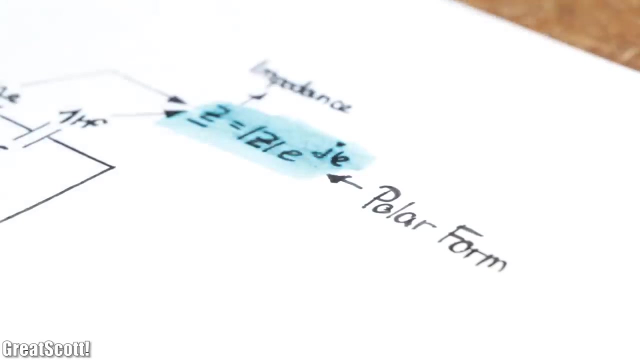 would only deliver wrong values, And thinking the phase angle would stay at 90 degrees is also incorrect. The solution is to turn both values into a complex impedance and calculating with that. This one is the polar form of the impedance, but also important for calculations. 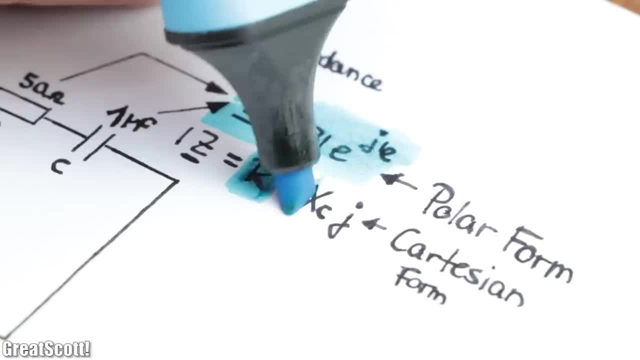 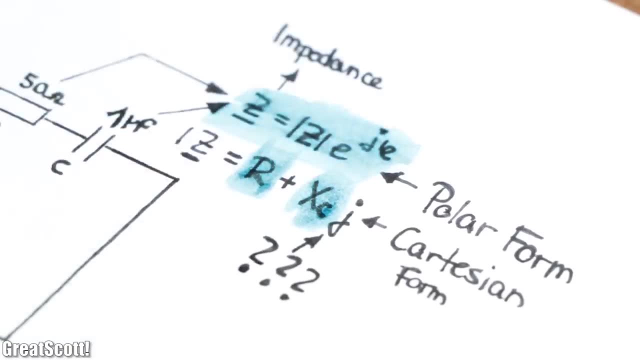 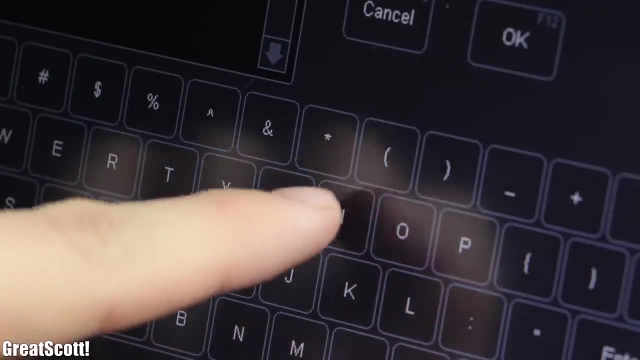 is the Cartesian form. In it we can see our known values for the resistance and reactance. But there's also a J. This J is actually the imaginary unit I of the imaginary number system, But since I usually refers to current in electronics, 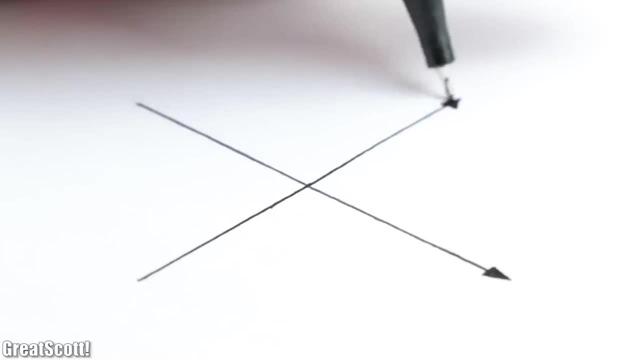 we stick to the J. If we would now draw a complex plane with the x-axis being the real axis and the y-axis being the imaginary number, we could now plot our resistance and reactance. The resistance is obviously real, so we go with a value of 50 ohms to the right. 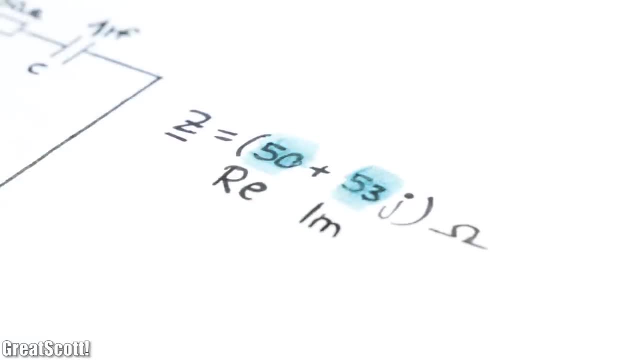 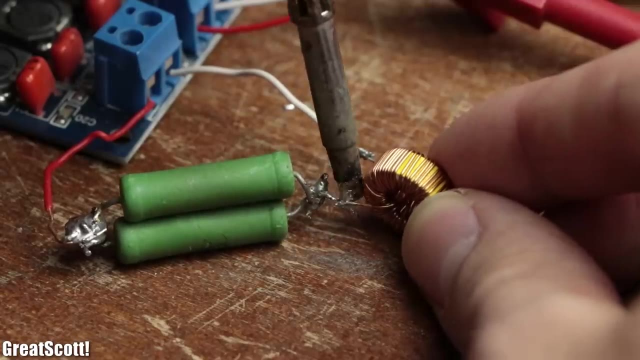 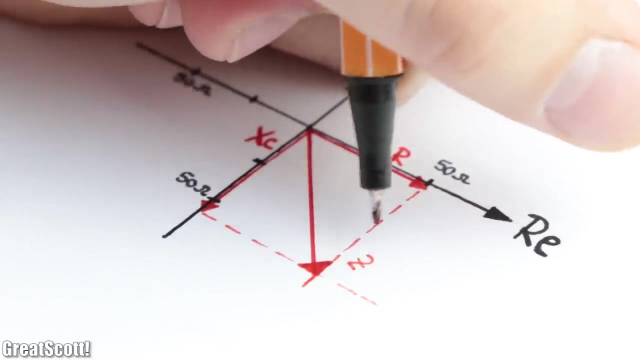 The reactance, however, is imaginary, meaning we go 53 ohms down. And, by the way, if we would use an inductor instead of the capacitor, the direction of the arrow would be inverted, so upwards. But anyway, the now emerging arrow is the impedance vector we've been looking for. 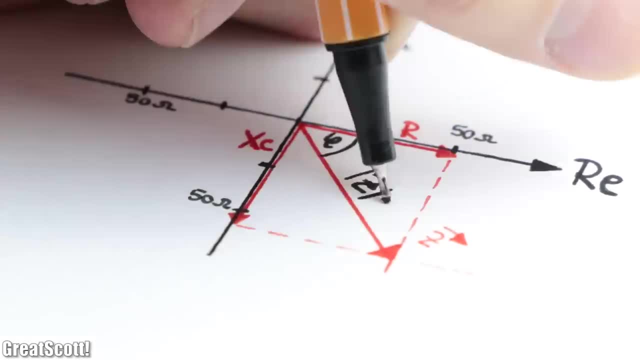 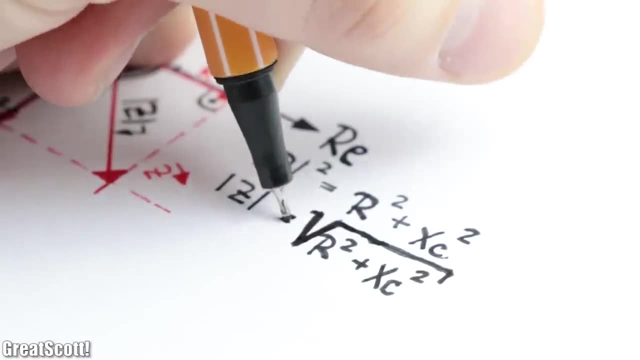 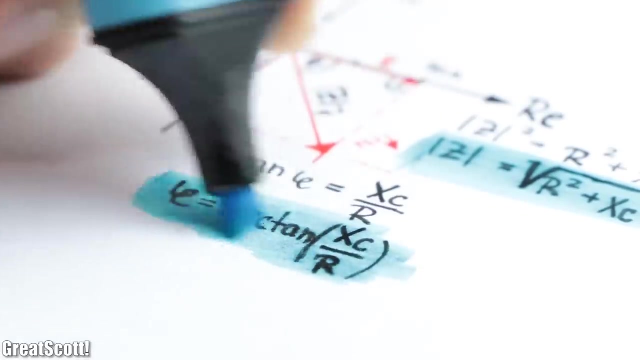 Its angle is required for the phase angle and its magnitude for the current calculation. So, according to simple trigonometry, the magnitude equals the root of r squared plus xc squared, and the phase angle is arctangent of xc divided by r. 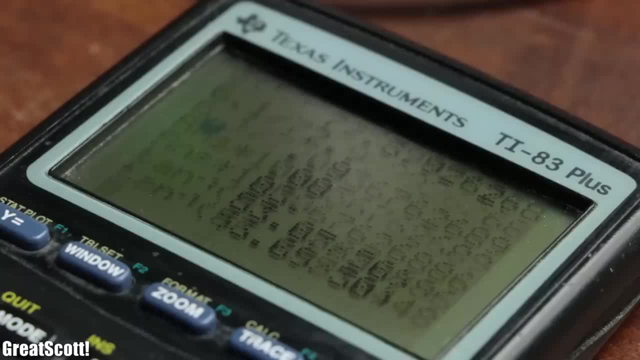 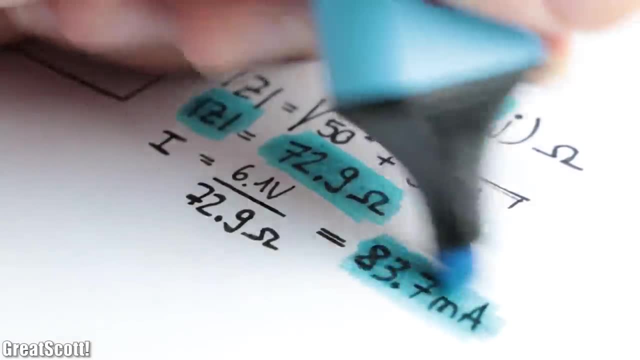 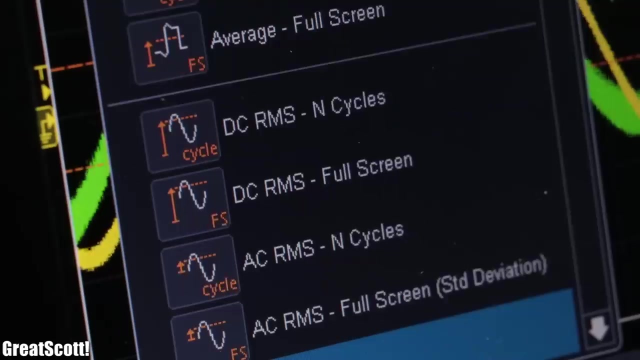 And by using my trusty old TI83+, I calculated a magnitude of 72.9 ohms, which equals a current flow of 83.7 milliamps and a phase angle of 46.7 degrees, By measuring the corresponding values at the practical circuit.